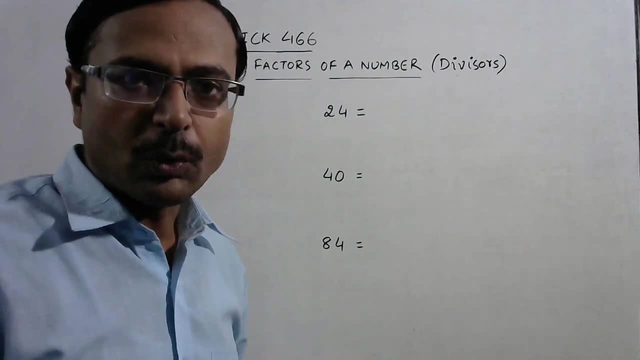 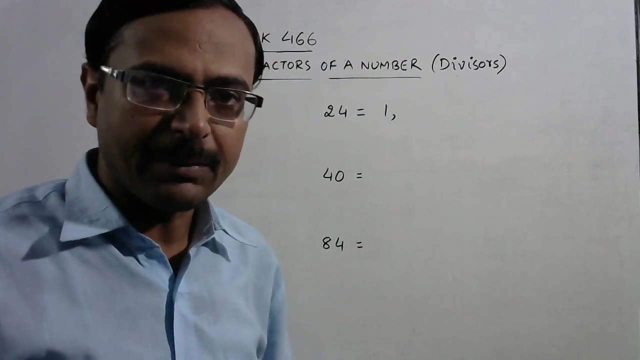 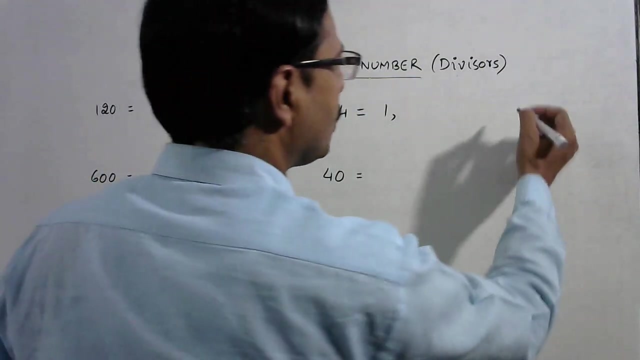 separately, by separating them out with commas. So we will start with 1, because 1 is a factor of, or a divisor of, everything. On the other side, 24 divided by 1 gives you 24.. So 24 will be the last factor. Now move from 1,. 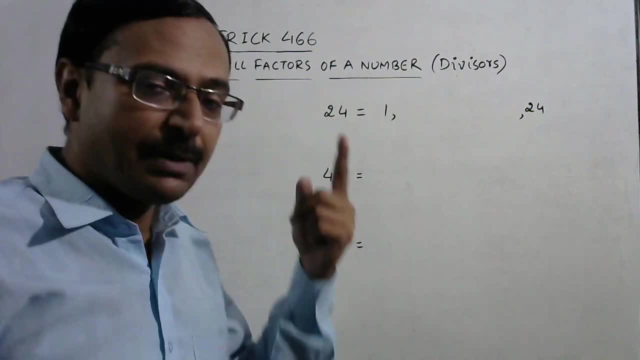 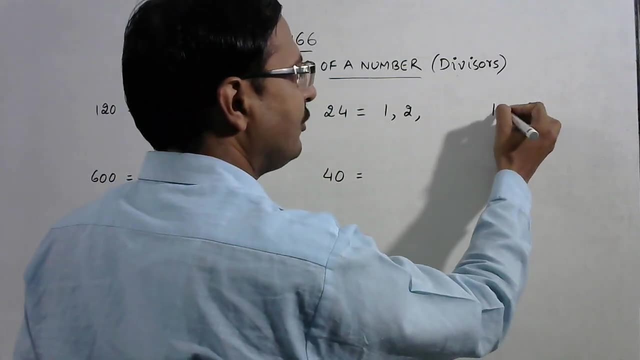 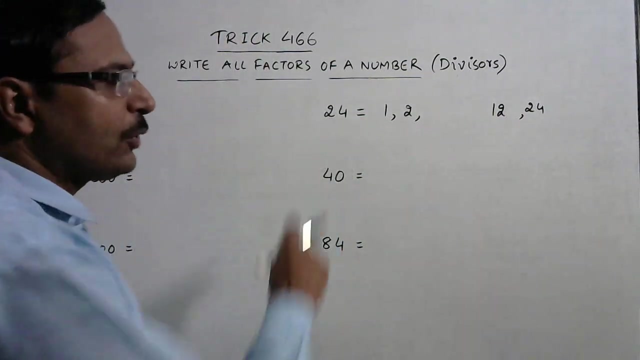 obviously 24 is an even number, So this will be divisible by 2.. So 2 will be a divisor, and 24 divided by 2 is 12.. So 12 will be the factor previous or preceding to 24.. Now 24. 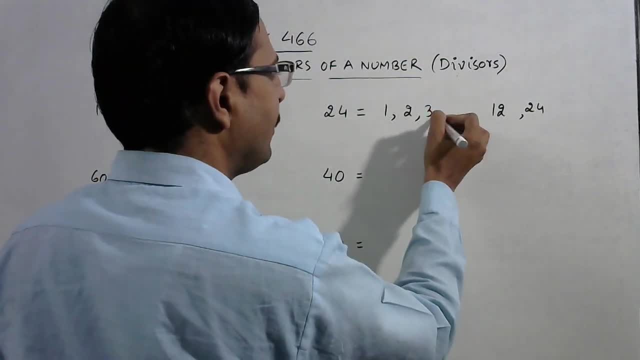 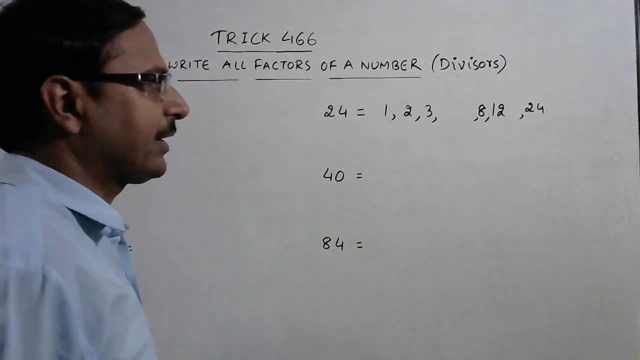 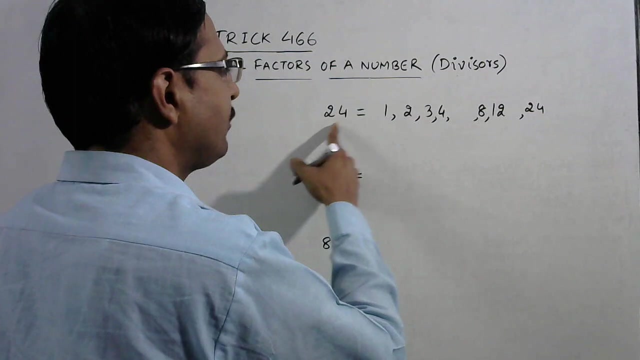 occurs in the table of 3 also. So 3 and 24 divided by 3 is 8.. So we have 8 also as the factor. Again we have 4.. 4 into 6 is 24.. So 4 is a factor and 24 divided by 4 is 6.. So 6 will also be a. 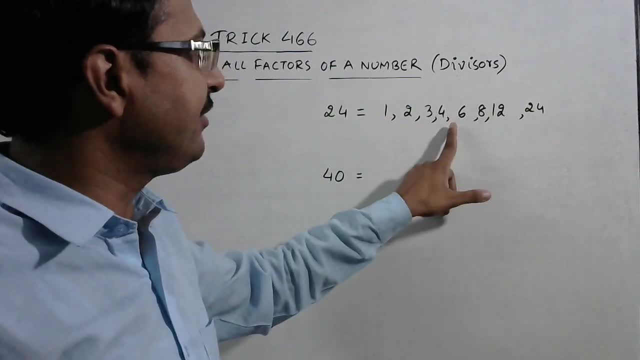 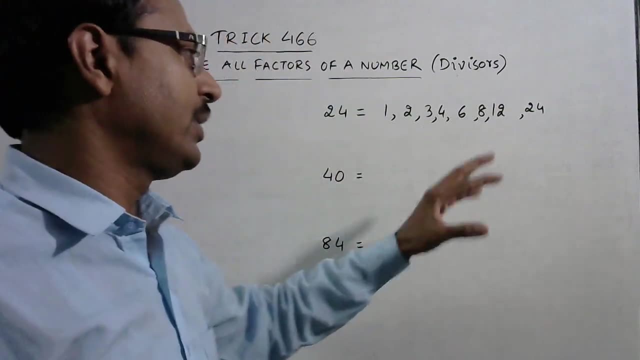 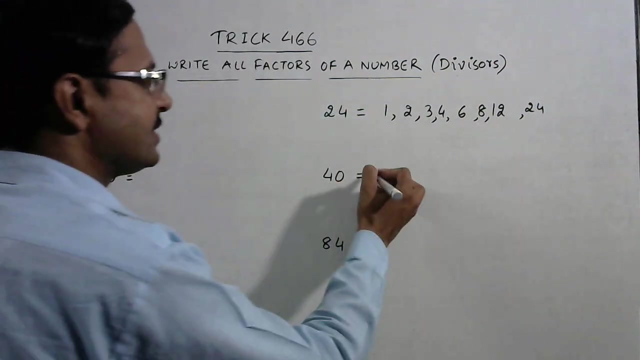 factor Now between 4 and 6, we have only 5, and 5 does not divide 24.. So we have completed all the factors of 24.. 4. So there are 8 factors: 1, 2, 3, 4, 6, 8,, 12 and 24.. Likewise, let us take 40. So we will start. 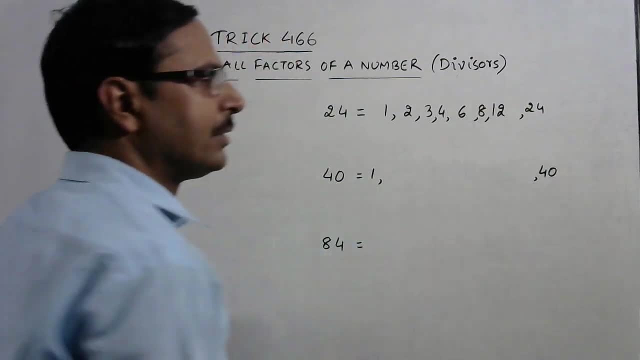 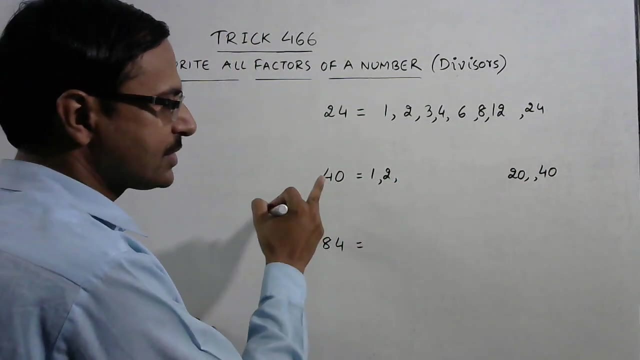 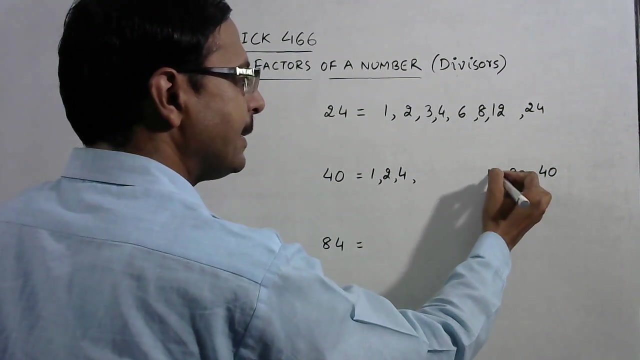 with 1, end with 40, 2. obviously it will be there. So 20, 3 is not a factor because 40 does not occur in the table of 3.. Obviously it comes in the table of 4.. So 4 ends up 40, 5 also 5,. 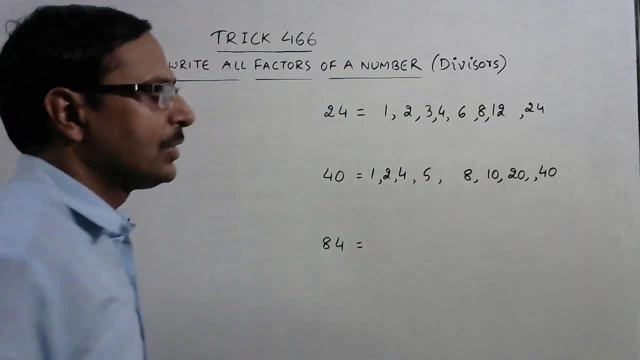 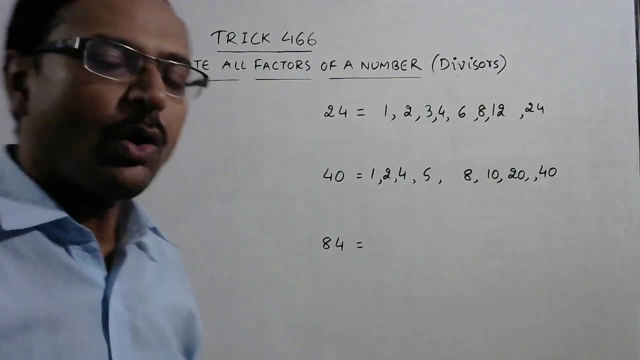 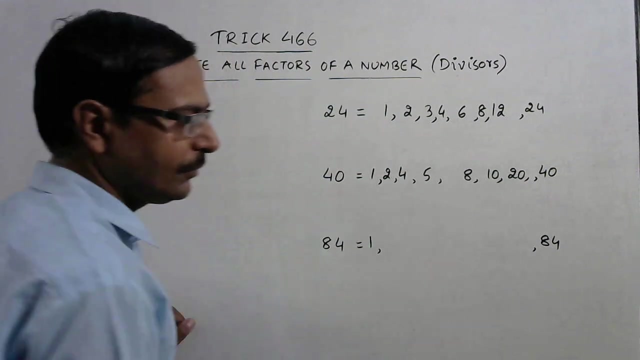 5 ends up 40. Now between 5 and 8, we have 6 and 7,. 6 does not divide 40 and 7 does not divide 40. So we have completed all the factors of 40.. 84, say 1 and 84, 2, 84 divided by 2 is 42,. 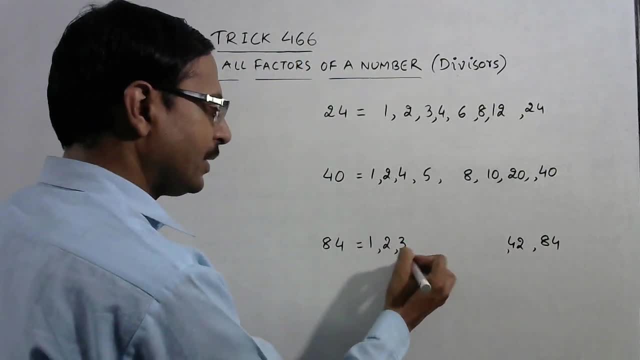 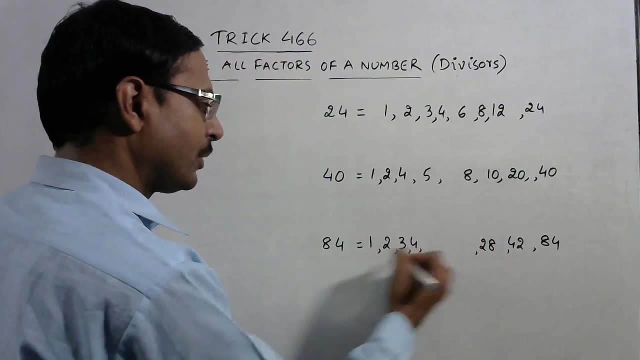 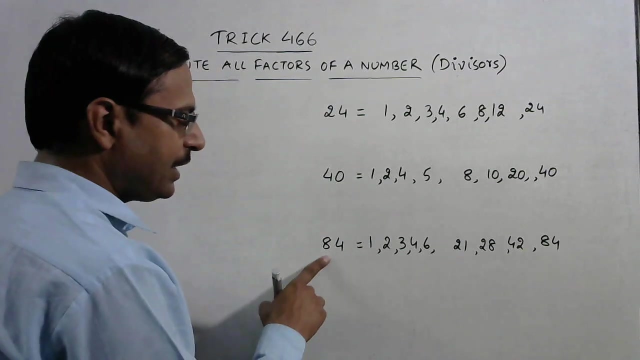 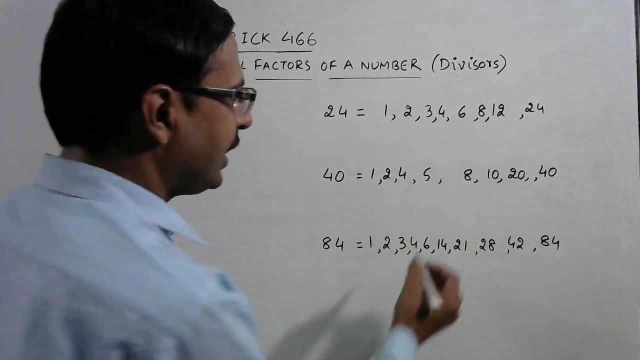 2, 3, 84 divided by 3 is 28,. 2, 4, 84 divided by 4 is 21,. 6, 84 divided by 6, 14, and between 6 and 14, we have 7, it divides. 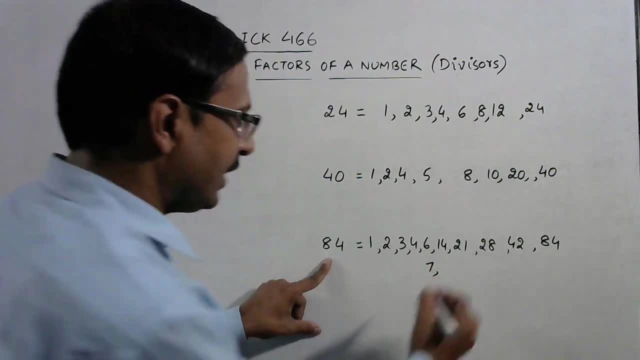 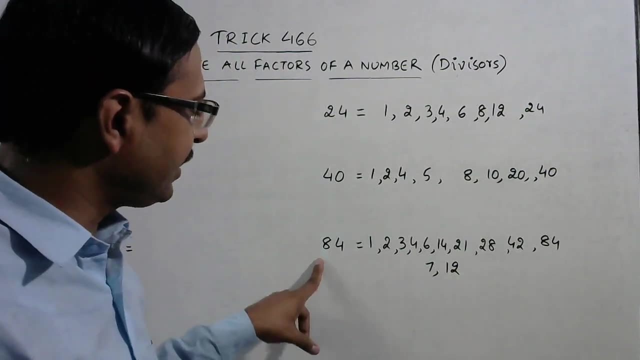 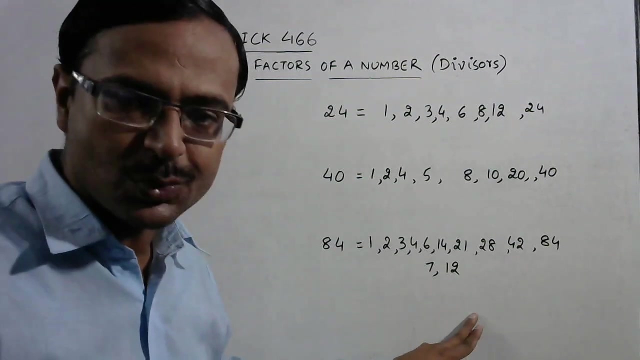 So 7 will also be there, So 12 and between 7 and 12, we have 8, it does not divide 84,. 9 does not divide 84,. 10,, 11, no number divides 84 between 7 and 12.. So we have 1,, 2,, 3,. 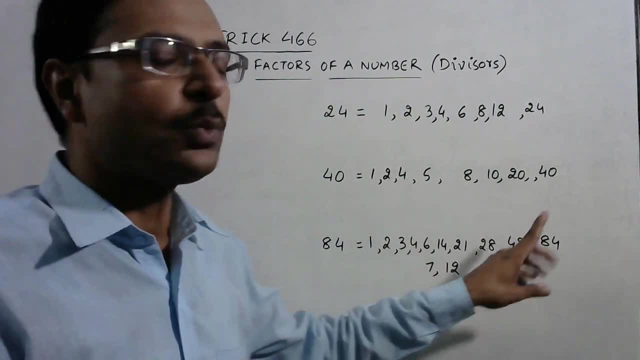 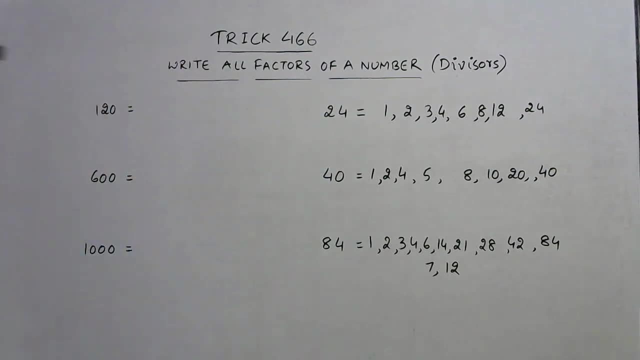 4,, 6,, 7,, 12,, 14,, 21,, 28,, 42 and 84 as the divisors or the factors of 84.. Let us have some larger numbers. This time we are taking up 120.. Say 1,. I will write 120 here. 2,. 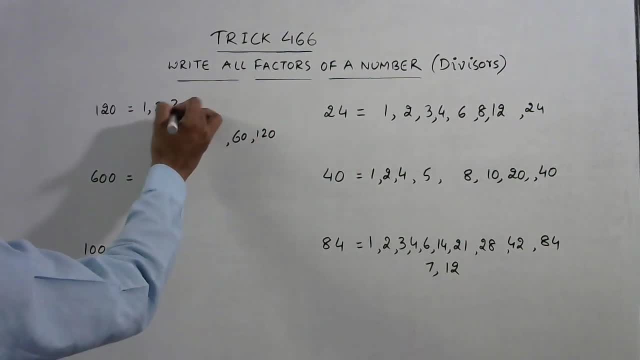 60, 3, 40. So we are narrowing this gap: 4, 30,, 5, 24,, 6, 20 and between 6 and 20, we have 8, 15,. 9 does not divide this, So 10, 12.. 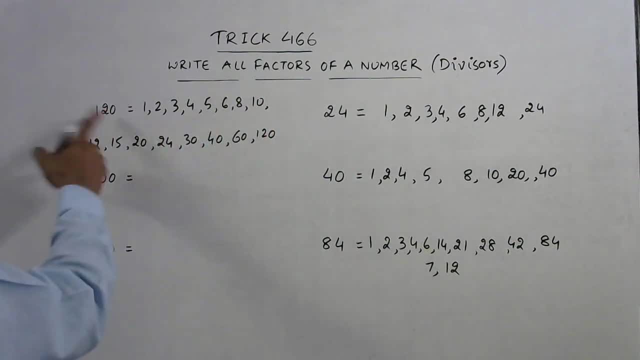 So between 10 and 12, we have 11,. it does not divide 120.. So the factors are 1, 2, 3, 4, 5, 6, 8, 10,, 12,, 15,, 20,, 24,, 30,, 40,, 60,, 120.. So in this method you do not need to consider the large. 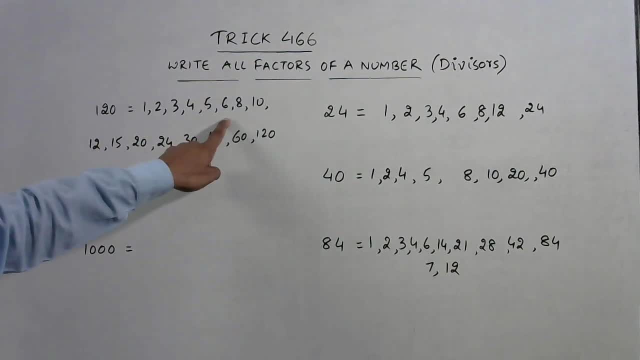 numbers. You can only consider the numbers which are smaller and find out the numbers which are larger by dividing this number with that number. Now let us have 600.. Say 1, 600, 2, 300,, 3, 200,, 4, 150.. So this gap is narrowing: 5, 120,, 6, 100.. So 7, it does not divide. 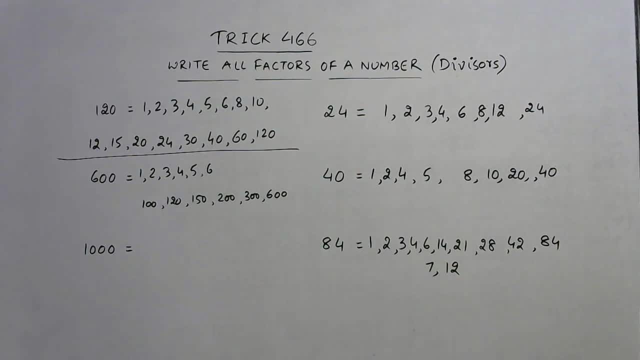 7 does not divide 600.. 8, 8, 7 is a 56. So 8, 7 is a 56.. So 40, 8, 5 is a 40. So 8, 70, 5 times 9, 9, 6 is a 54, 60. It does. 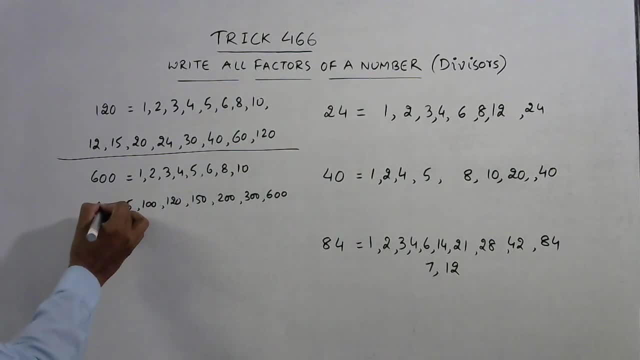 not divide. So we have 10, 60,. 11 does not divide this 12,. obviously it will divide 12,. 5 is a 60. So 12 and 50. 13,, 14,, 15, 40. Now see the gap, It is narrowed down. 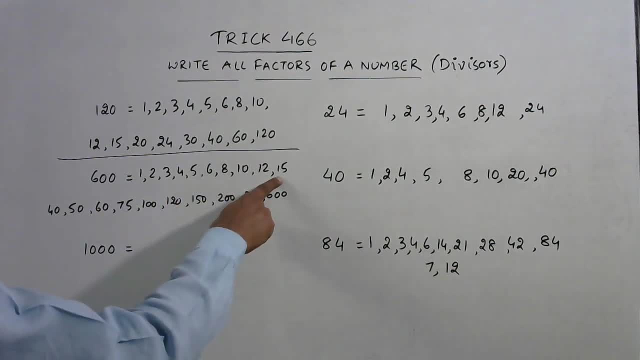 Now you can have more numbers from here: 15,, 16,, 17,, 18,, 19.. We have 20 also, So 20, it becomes 30. Now see the gap: 20, 30. So between them 21,, 22,, 23,, 24, they do not divide 600. So we have 25.. 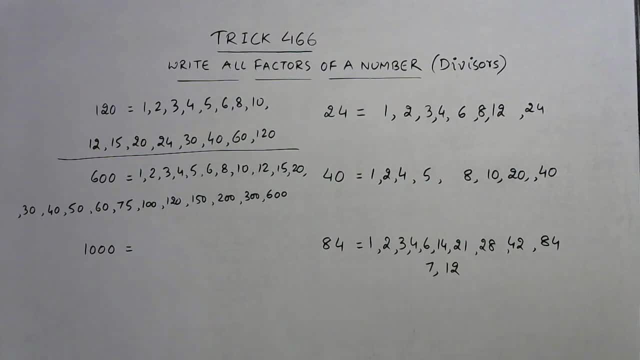 So yet another number: 25.. 25, 2 is a 50 and 4. So 24 and 25.. So obviously now, when we took that, 24 also divides 600.. So now we have written 24 also and 25 also, and obviously now there is no. 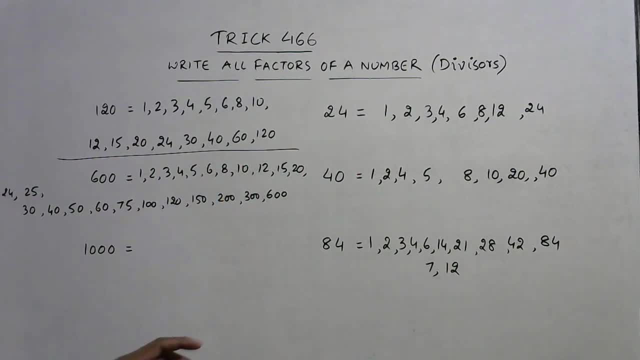 gap between the numbers. So we have completed all the factors and see the number of factors: 1 to 6, all numbers 8, 10, 12,, 15,, 20,, 24,, 25,, 30,, 40,, 50,, 60,, 75,, 100,, 120,, 150,, 200,, 300 and. 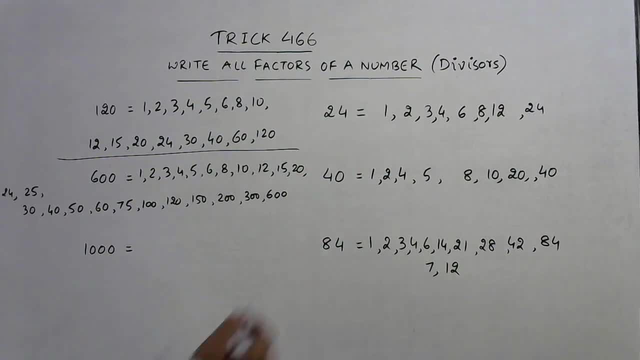 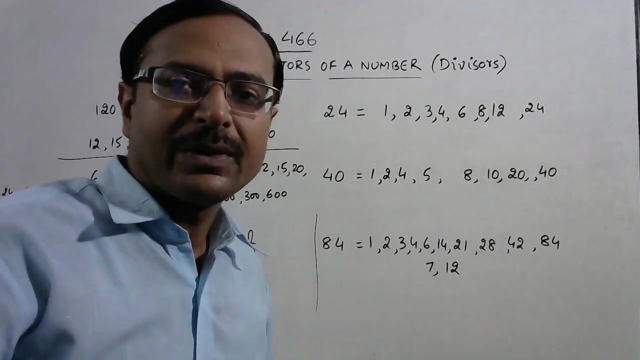 600.. Likewise, you can carry on with this number: 1000.. I will leave it for you and try out this number and find out all the divisors of 1000 by using this amazing method, which can be called a shortcut. So, students, through this method you will be able to find out all. 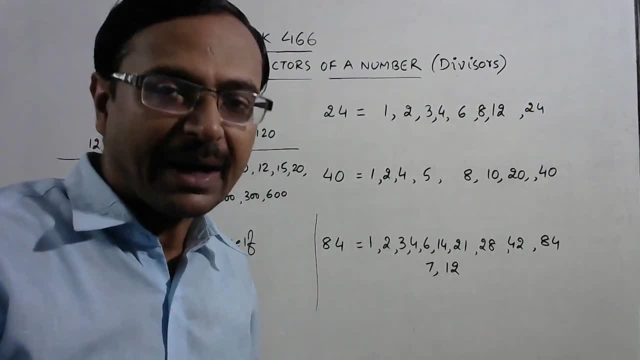 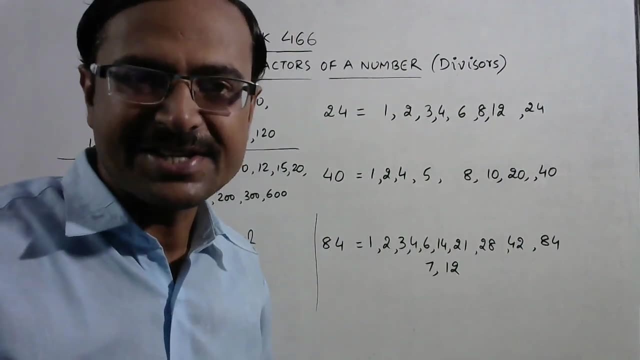 the factors of a given number and remember: practice makes a man perfect, So you need to practice the method in order to master it. So if you like the video, do share it and subscribe the channel.